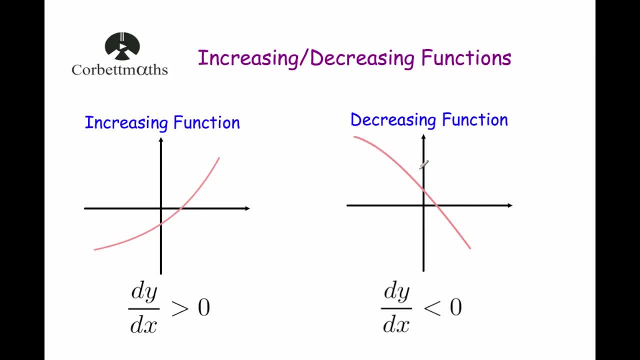 which is going downwards. so as the values for x are increasing, the values for y are decreasing and the gradient of the tangents will always be negative. so dy by dx will always be negative for a decreasing function. Some functions are increasing or decreasing for different. 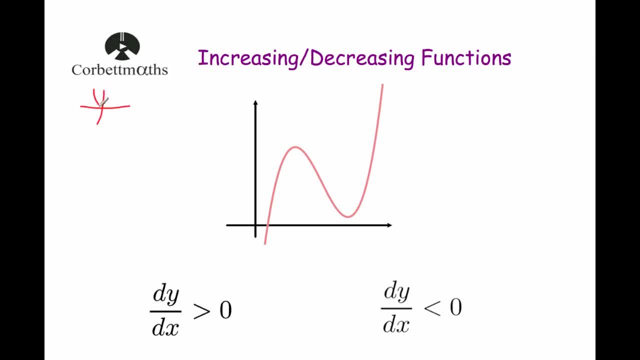 values of x. so if you think of a quadratic, obviously just something like that, you'll see it will be decreasing and then it will then become an increasing function. so here we've got a cubic and we can tell this because we've got the maximum point here, the minimum point here and for some. 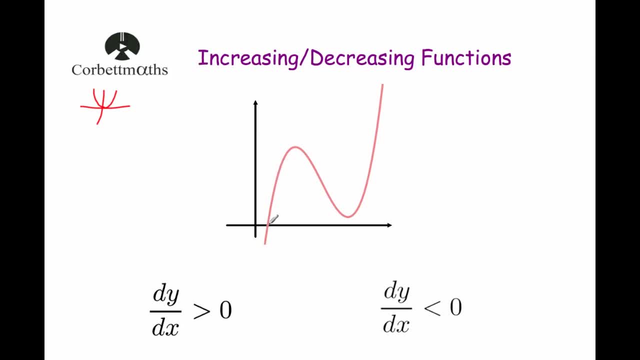 values of x, this cubic is increasing. so it's increasing here, increasing, increasing, increasing, increasing until you get to here. so for all these values of x, dy by dx is positive, then the function starts to decrease and it decreases all the way down to here. so, for these values of x, this is a 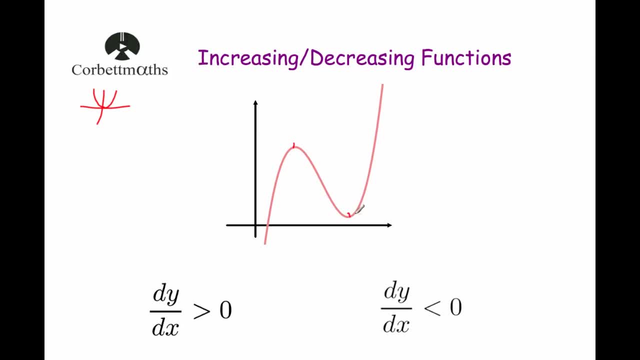 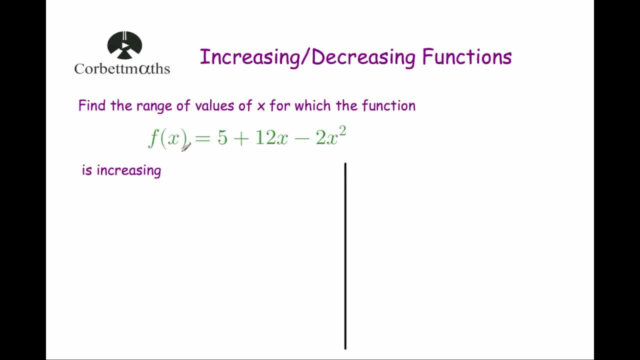 decreasing function, and then for all the rest of the values of x. so all these values of x, the gradient is positive, so it's increasing again. so this function, this cubic, is increasing, then decreasing and then increasing. okay, so our first example, our first example says: find the range of 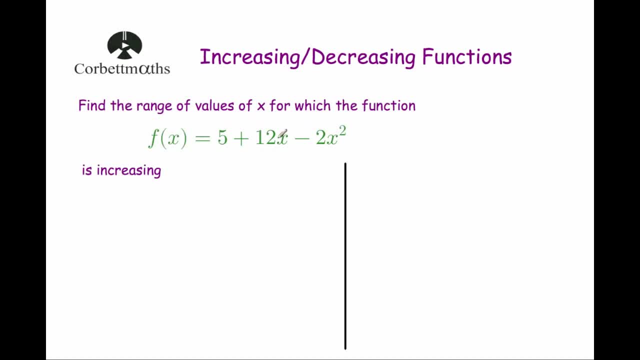 values of x, for which the function f of x equals 5 plus 12, x minus 2 x squared- is increasing. now we're going to solve this question using two different approaches. the first approach is just considering what the function is, and then the second approach is just considering what the 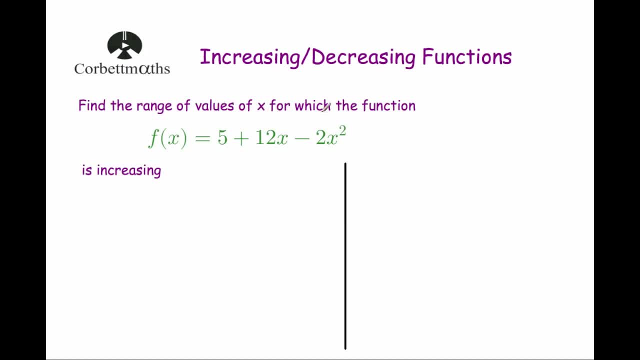 function looks like and then working out the values of x for whenever the function is increasing. so looking at the graph and working that out. and the second approach is just by considering that dy by dx is positive, that the gradient is positive for an increasing function. so we'll just differentiate. 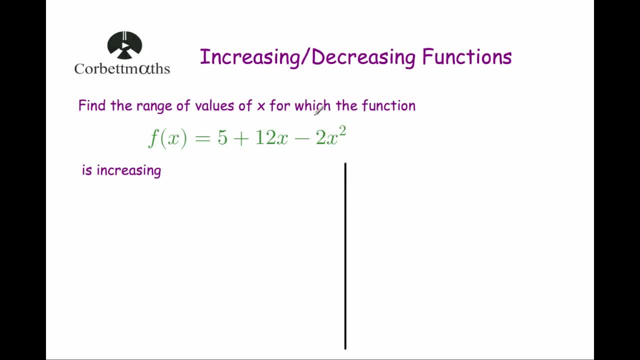 it and solve that inequality. so first of all let's consider what the function looks like. so it's 5 plus 12 x minus 2 x squared, so it's a negative x squared. so it's going to be an n-shaped parabola, so it's a quadratic, but it's a negative one, so it's going to look something like that: 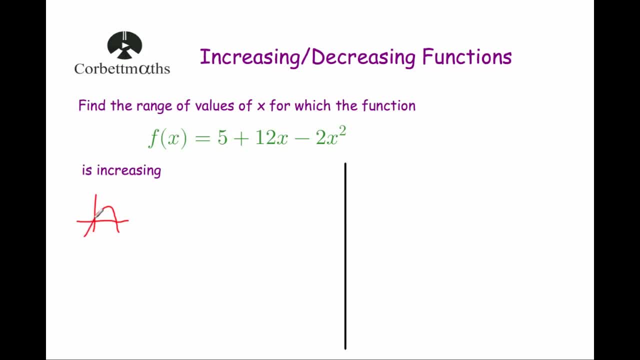 and we know that the function is increasing. so we're going to solve this question using two different approaches. so we'll just consider what the function is and then we're going to solve this. function is increasing, increasing, increasing, increasing up until the stationary point and then, after the stationary point, it'll be decreasing, decreasing, decreasing. so you know that all the 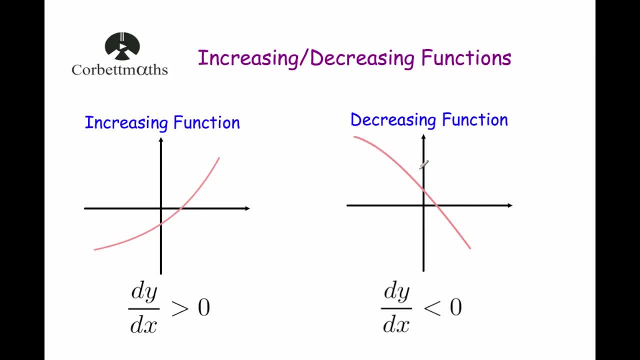 which is going downwards. so as the values for x are increasing, the values for y are decreasing and the gradient of the tangents will always be negative. so dy by dx will always be negative for a decreasing function. Some functions are increasing or decreasing for different. 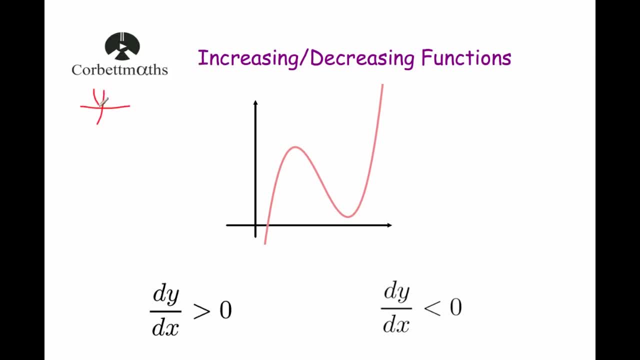 values of x. so if you think of a quadratic, obviously just something like that, you'll see it will be decreasing and then it will then become an increasing function. So here we've got a cubic and we can tell this because we've got the maximum point here, the minimum point here. 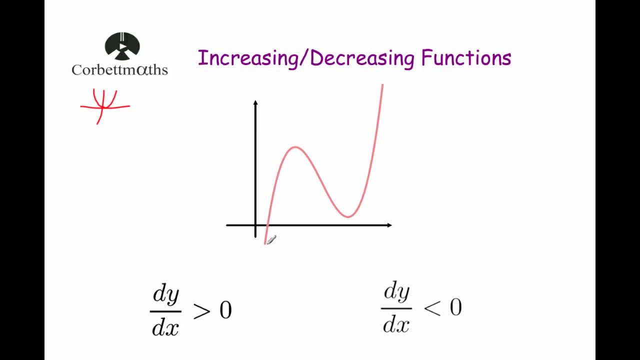 and for some values of x, this cubic is increasing. so it's increasing here, increasing, increasing, increasing, increasing until you get to here. So for all these values of x, dy by dx is positive, Then the function starts to decrease and it decreases all the way down to here. 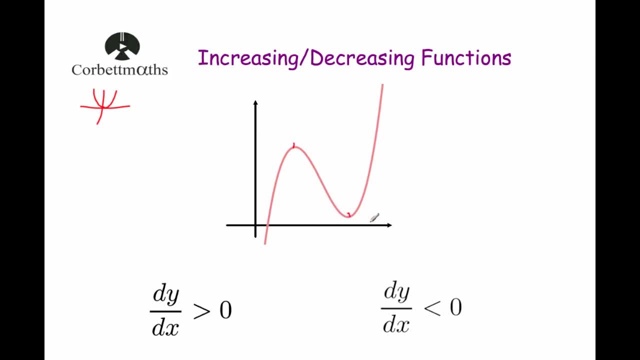 so for these values of x, this is a decreasing function- and then for all the rest of the values of x. so all these values of x, the gradient is positive, so it's increasing again. So this function, this cubic, is increasing, then decreasing and then increasing. Okay, so our 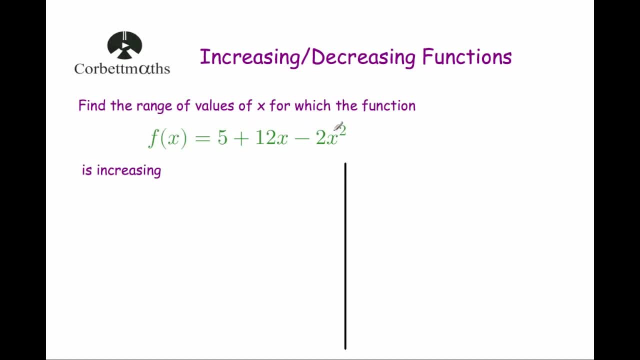 first example. Our first example says: find the range of values of x, for which the function f of x equals 5 plus 12x minus 2x squared, is increasing. Now we're going to solve this question using two different approaches. The first approach is just considering what the function looks like. 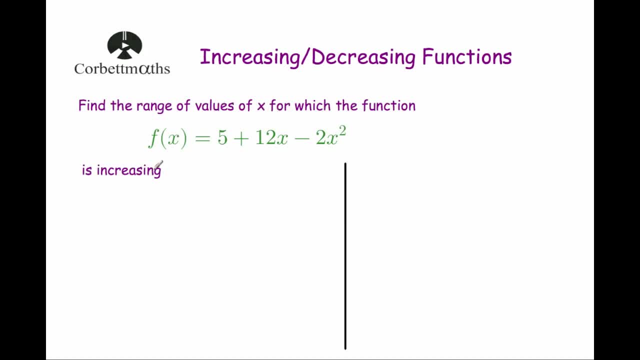 and then working out the values of x for whenever the function is increasing. So looking at the graph and working that out. And the second approach is just by considering that dy by dx is positive, that the gradient is positive for an increasing function. so we'll just 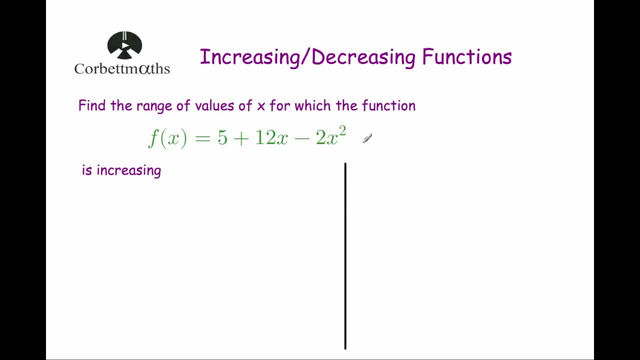 differentiate it and solve that inequality. So first of all let's consider what the function looks like. So it's 5 plus 12x minus 2x squared, so it's a negative x squared, so it's going to be an n-shaped parabola, So it's a quadratic, but it's a negative one, so it's going to look something. 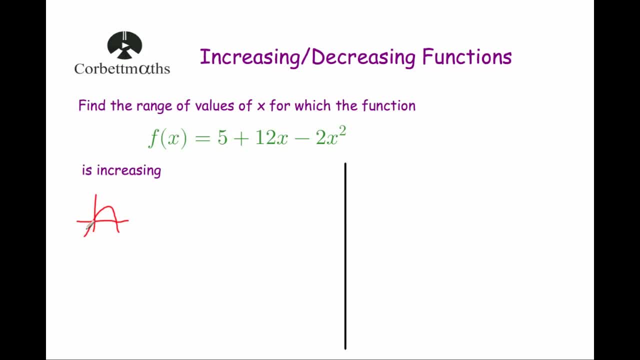 like that, And we know that this function is increasing, increasing, increasing, increasing and then, after the stationary point, it'll be decreasing, decreasing, decreasing. So we know that all the values of x left off the stationary point will give us an increasing function. So 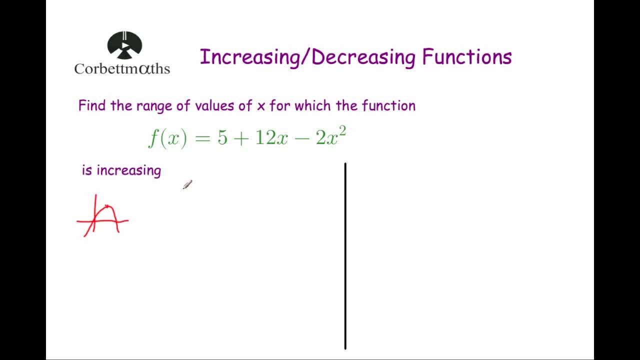 let's find the coordinates of the stationary point. So we know that at a stationary point the gradient is equal to 0, so dy by dx is equal to, and differentiating this we'll differentiate in 5, 0.. Differentiating 12x would be 12, and differentiating minus 2x squared we'll bring in. 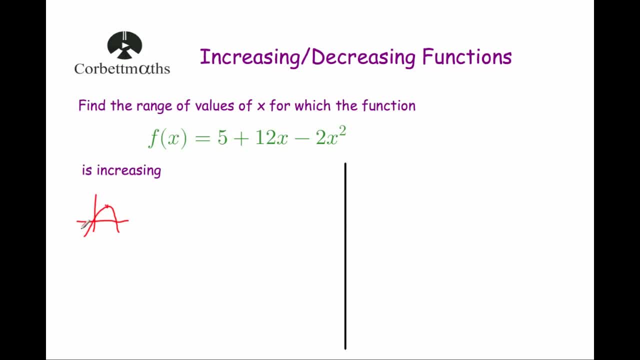 values of x left off the stationary point will give us an increasing function. so let's find the coordinates of the stationary point. so we know that at a stationary point the gradient is equal to zero. so dy by dx is equal to and differentiate this, we'll differentiate in five, zero differentiate. 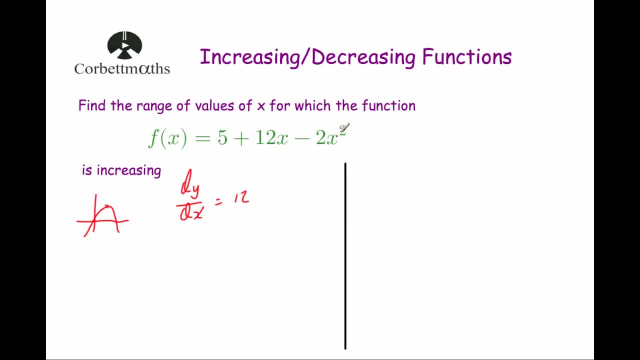 in twelve x would be twelve and differentiate in minus two x squared, we'll bring in the two down minus four x and reducing the part by one will just be one. now we know that's equal to zero. so zero equals twelve minus four x, and adding four x to both sides will give us four x equals twelve. 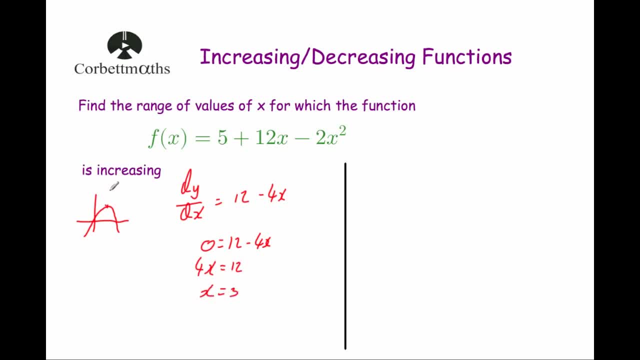 dividing by four, we give us, x equals three. so at the stationary point the x coordinate is equal to three. now we don't actually need to know what the y coordinate is, because we're only interested in the values of x, for which the function is increasing. and we can already tell now that every 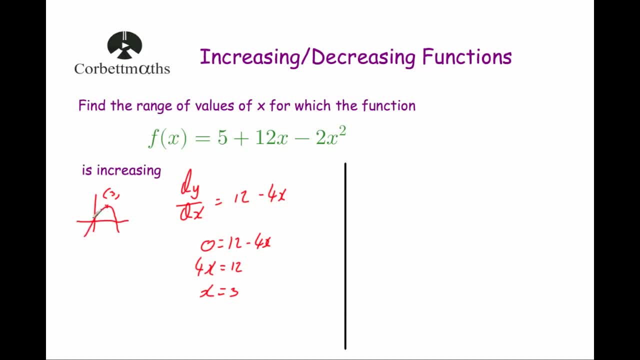 x value less than three would give you an increasing function. um, i do know that the y coordinate is 23, so i'm just going to write that in anyway. okay, but, as i said, we're trying to find the values for x, for which the function is increasing now. 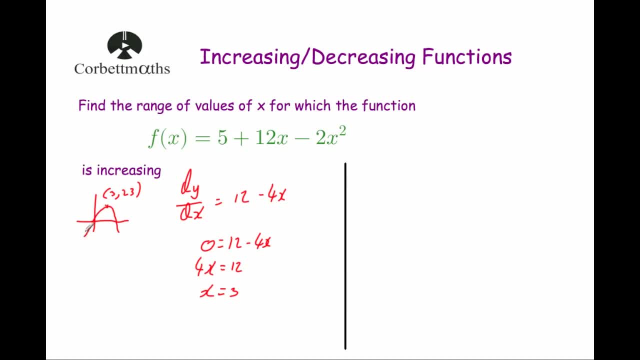 everywhere to the left of the stationary, if the gradient is positive, it's increasing, increasing, increasing, increasing. so x is less than three would be our answer. all the values of x less than three would give us an increasing function and then bigger than three would be a decreasing. 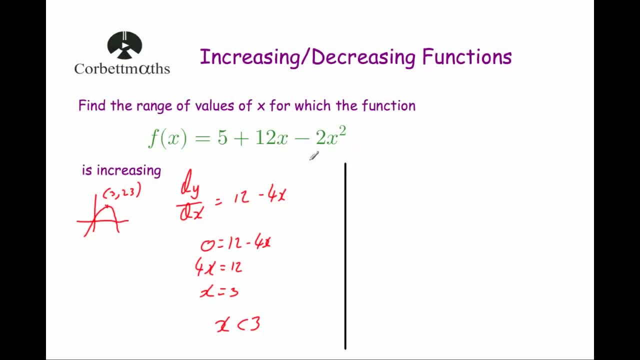 function okay. our second approach is just by considering the dy by dx. we know that it's increasing, so we can say that dy by dx is positive. it's bigger than zero. so if we want to find this, what we're going to do is we're just going to differentiate, which we've done. 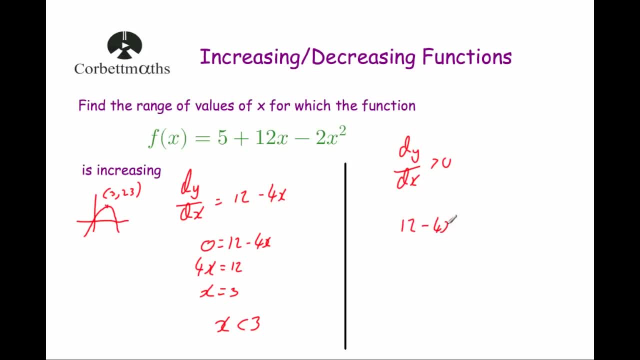 dy by dx is equal to 12 minus 4x, and for an increasing function it's going to be bigger than 0.. now we can just solve this in equally, so adding 4x to both sides would give you 12 is bigger than. 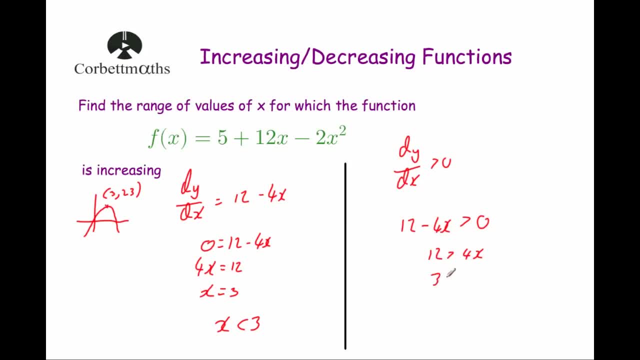 4x. dividing both sides by 4 would give you 3 is bigger than x and just right another way around 3 and that's it. as you can see, both approaches give you the same answer. some students prefer to use this approach: just considering what the graph looks like and then working out when it's. 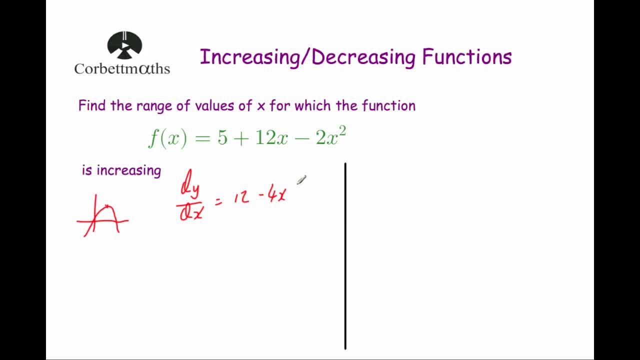 the 2 down will be minus 4x, and reducing the part by 1 will just be 1.. Now we know that's equal to 0, so 0 equals 12 minus 4x, and adding 4x to both sides will give. 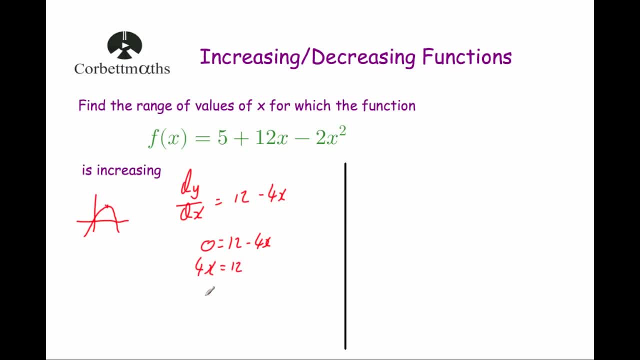 us 4x equals 12, dividing by 4 will give us x equals 3.. So at the stationary point the x coordinate is equal to 3.. Now we don't actually need to know what the y coordinate is, because we're only interested in the values of x, for which the function is increasing, and we can 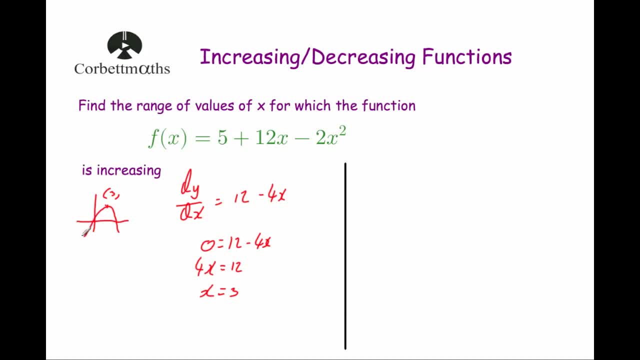 already tell now that every x value less than 3 would give you an increasing function. I do know that the y coordinate is 23,. so I'm just going to run through that. So we know that the y coordinate is 23,. so we know that the y coordinate is 23,. so we know that the y coordinate is 23,. so we know that. 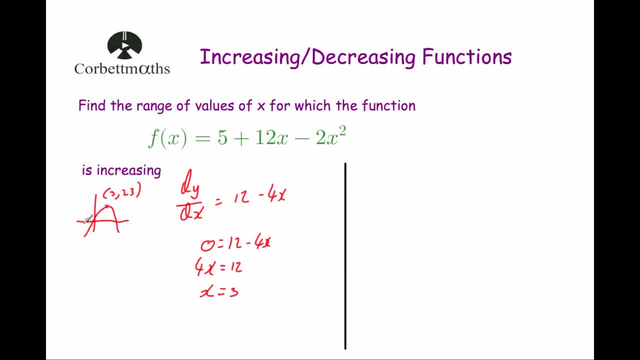 that it is anywhere, Okay. but, as I said, we're trying to find the values for x, for which the function is increasing now everywhere to the left of the stationary. if the gradient is positive, it's increasing, increasing, increasing, increasing. so x is less than 3 would be our. 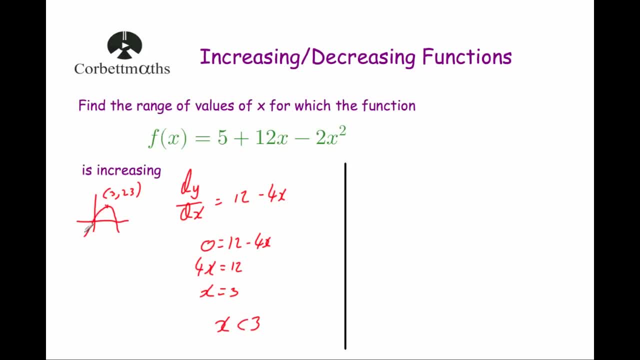 answer: All the values of x. less than 3 would give us an increasing function and bigger than 3 would be a decreasing function. Okay, our second approach is just by considering the dy by dx. we know that it's increasing, so we can say that dy by dx is. 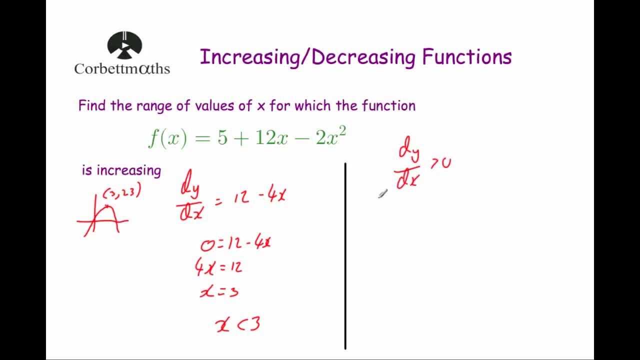 positive, it's bigger than zero. so if we want to find this, what we're going to do is we're just going to differentiate, which we've done. dy by dx is equal to 12 minus 4x, and for an increasing function it's going to be bigger than zero. now we can just solve this inequality, so adding 4x to 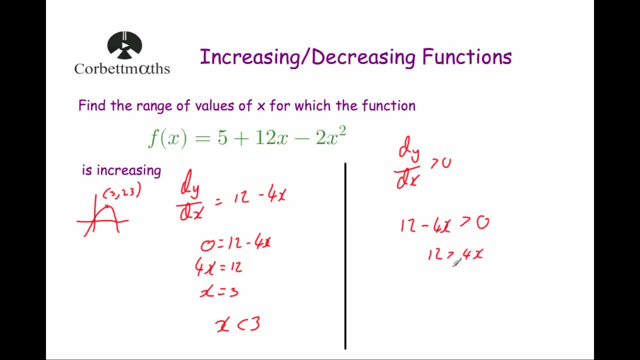 both sides would give you 12 is bigger than 4x. dividing both sides by 4 would give you 3 is bigger than x, and just writing that the way around would be: x is smaller than 3 and that's it. as you can see, both approaches give you the same answer. some students prefer to use this approach just. 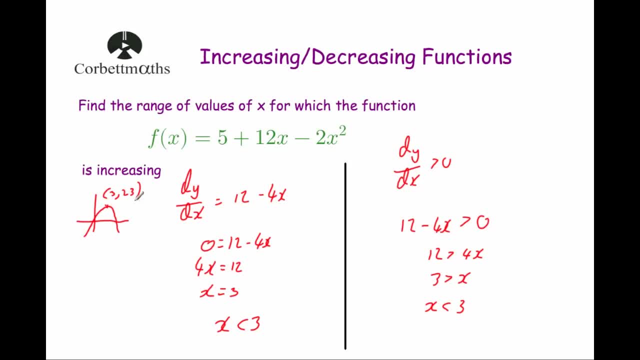 considering what the graph looks like and then working out when it's increasing. some students just like using the fact that if it's an increasing function, dy by dx is positive and then solving that inequality. okay, let's have a look at a function which is a bit more complicated than 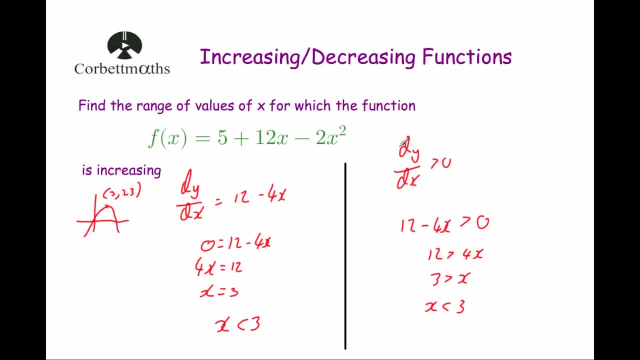 increasing. some students just like using the fact that if it's an increasing function, dy by dx is positive and then solving that inequality. okay, let's have a look at a function which is a bit more complicated than a quadratic. so our cubic. and so here we've got our cubic and the question says: 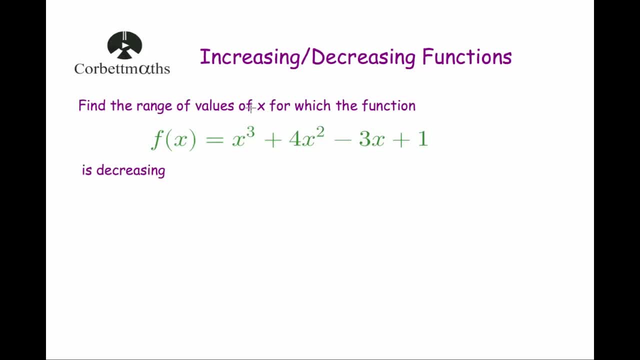 find the range of values of x for which the function. the range of values for x, for which the function f of x equals x cubed plus 4x squared minus 3x plus 1, is decreasing. so this time we want to find when this function is. 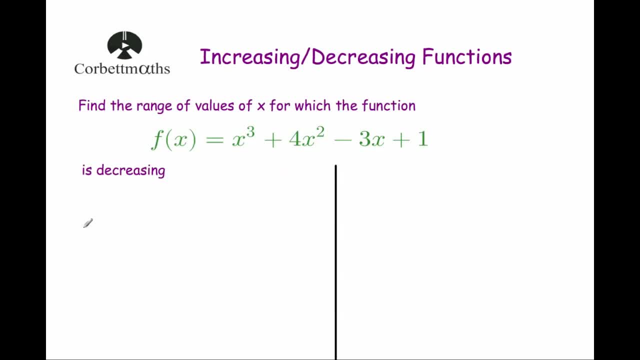 decreasing. again, we're going to use our approach where we consider what the graph looks like, the function looks like, and we'll solve it that way, and then we'll use our second approach by just knowing that, for a decreasing function, dy by dx would be less than zero. okay, so our first approach. 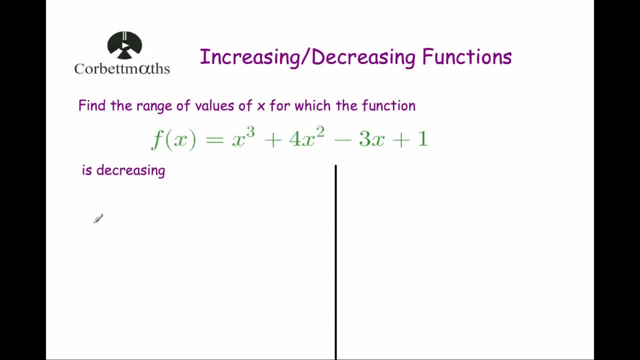 is considering what the function looks like. so we have got a cubic, so it's going to look, and it's an x cubed positive one, so it's going to go up and then down and then up again, something like that, and i'm just going to put in the x. 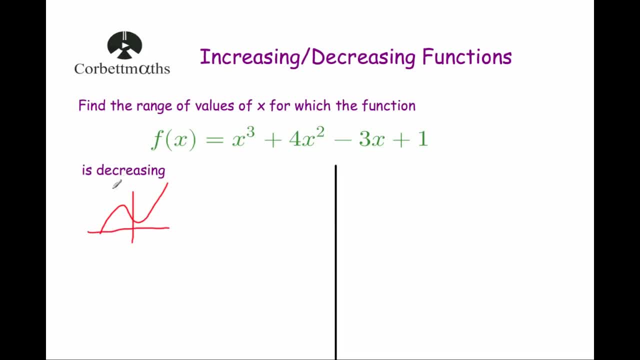 z's something like that, and we're trying to find when the function is decreasing. so let's have a look at this function: it's increasing, increasing, increasing, increasing, increasing to the first stationary point, and then it's decreasing, decreasing, decreasing to the second stationary point and then increasing again. so it's this section that we're interested in and 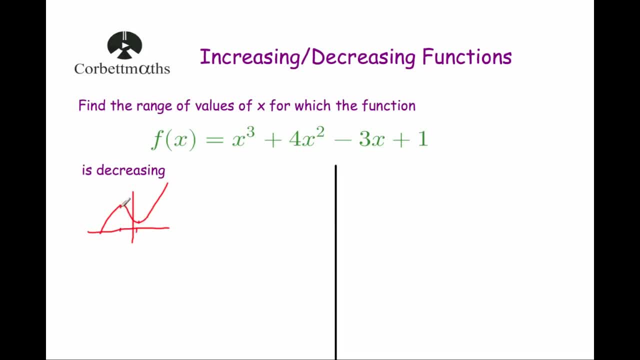 it would be the values for x between the two stationary points, because it's decreasing from the first stationary point down to the second stationary point. okay, so we need to find the coordinates of these two stationary points. so we know that for dy by dx, we're equal. 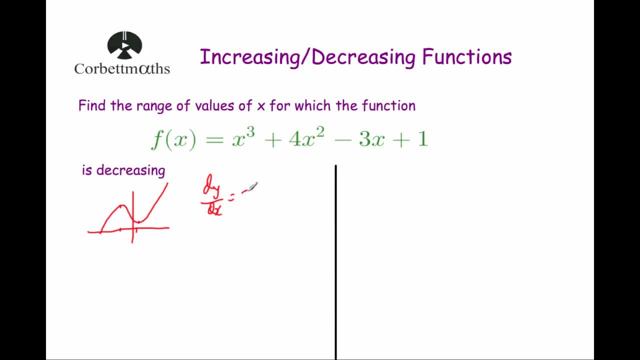 zero at a stationary point. so let's differentiate, so that'll be three. differentiating x cubed will be 3x squared, plus differentiating 4x squared we'll bring the power down, that'd be 8x, and then to the power of one. so we'll just write 8x and differentiating minus 3x would be minus three. 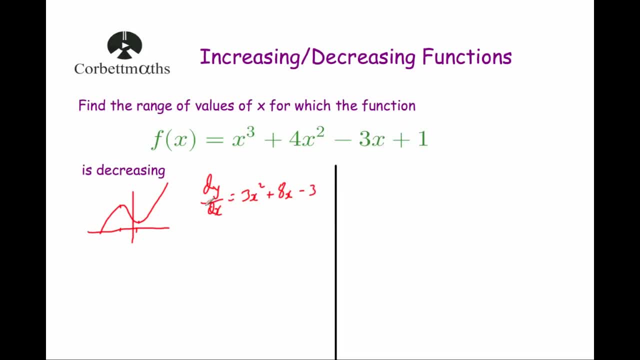 and differentiating zero would be, or differentiating one would be zero. so dy by dx is equal to 3x squared plus 8x minus three. now, at these stationary points, we know that the gradient is equal to zero here and here, so we're going to put that's equal to zero. so zero equals 3x squared plus 8x minus. 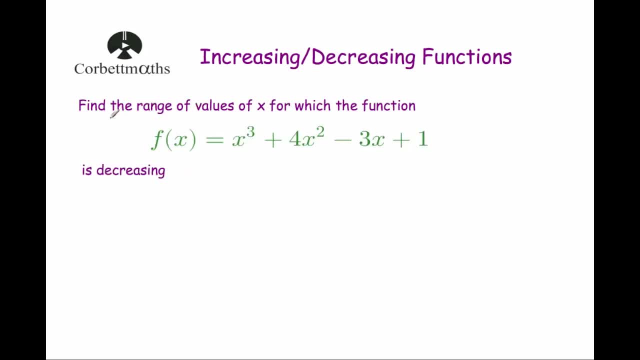 a quadratic, so a cubic. and so here we've got our cubic and the question says: find the range of values of x for which the function, the range of values for x, for which the function f of x equals x cubed plus 4x squared minus 3x plus 1- is decreasing. so this time we want to find when this function is decreasing. 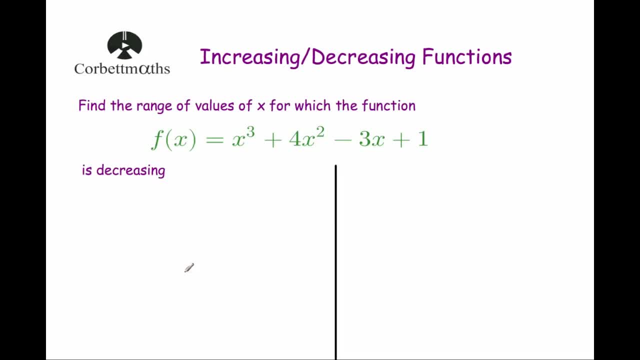 again, we're going to use our approach where we consider what the graph looks like, the function looks like, and we'll solve it that way. and then we'll use our second approach by just knowing that for a decreasing function, dy by dx would be less than zero. okay, so our first approach is considering: 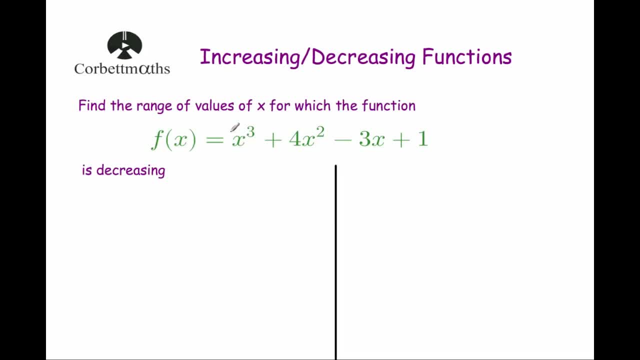 what the function looks like. so we have got a cubic, so it's going to look, and it's an x cubed positive one, so it's going to go up and then down and then up again, something like that, and i'm just going to put in the axes something like that. 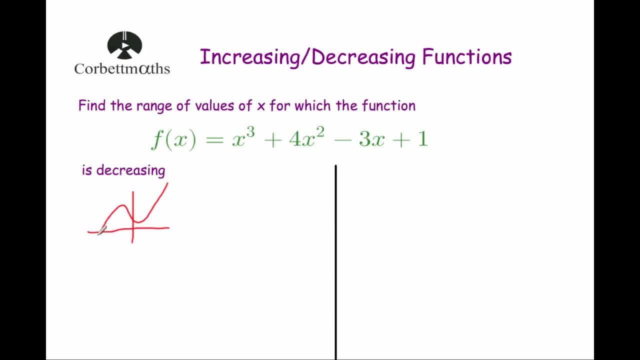 and we're trying to find when the function is decreasing. so let's have a look at this function: it's increasing, increasing, increasing, increasing, increasing to the first stationary point and then it's decreasing, decreasing, decreasing to the second stationary point, then increasing again. so it's this section that we're interested in, and it would be the values for x between the two. 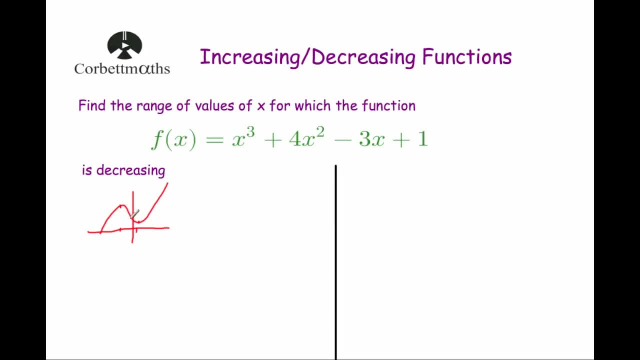 stationary points because it's decreasing from the first stationary point down to the second stationary point. okay, so we need to find the coordinates of these two stationary points. so we know that for dy by dx will equal zero at a stationary point, and we're going to find the 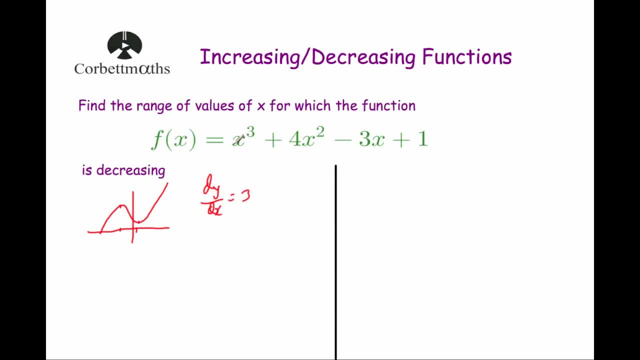 point. so let's differentiate, so that'll be three. differentiating x cubed will be 3x squared plus differentiating 4x squared, we'll bring the power down, that'd be 8x, and then to the power of one. so we'll just write 8x and differentiate. minus 3x will be minus three and differentiate in zero. 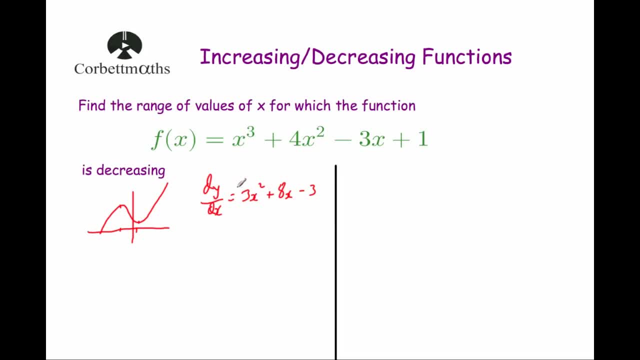 will be, or differentiate one will be zero. so dy by dx is equal to 3x squared plus 8x minus three. now, at these stationary points, we know that the gradient is equal to zero here and here. so we're going to write the value of x squared plus 8x minus three. so let's factorize this and find the. 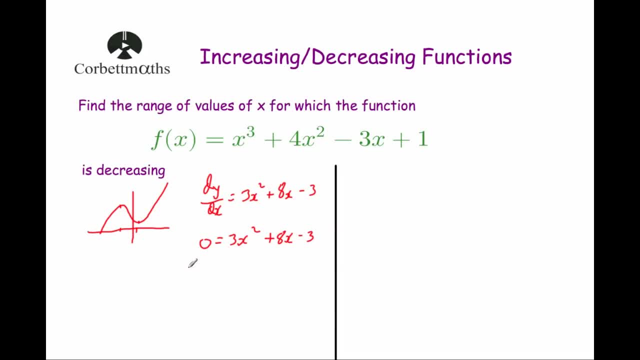 two values for x, for whenever the gradient is equal to zero. so zero equals. i'm factorizing 3x in one bracket and x in another. now we want the two numbers to times together to be negative three so, and we want, whenever we expand it, to get an 8x, uh, in the middle of positive 8x. so i'm going to. 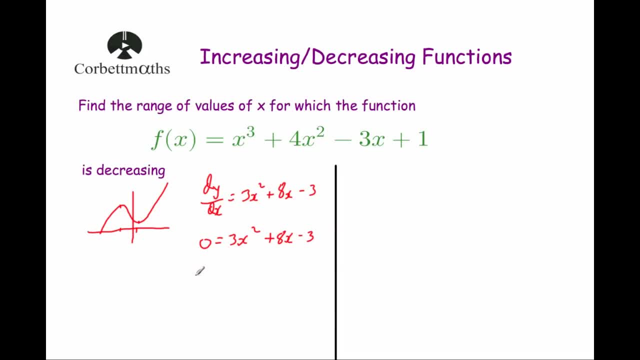 three. so let's factorize this and find the two values for x, for whenever the gradient is equal to zero. so zero equals. i'm factorizing 3x in one bracket and x in another. now we want the two numbers to times together to be negative three, so, and we want, whenever we expand it, to get an 8x. 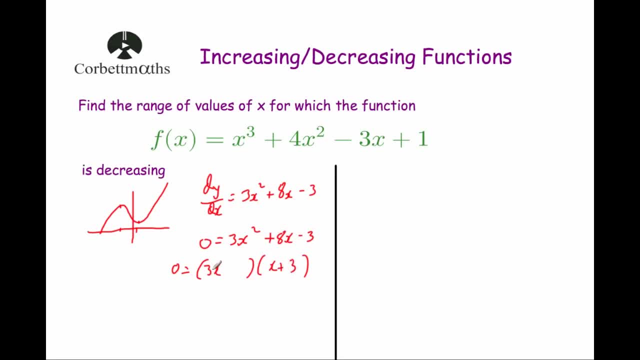 in the middle of positive 8x. so i'm going to put a plus three over there, so that will give me 9x. so i'm going to put a plus three over there, so that will give me 9x and i'm going to put a plus. 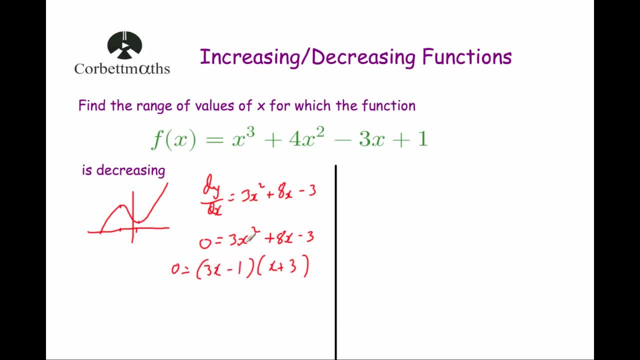 then a minus one here, and let's just test that. so 3x times x is 3x. squared 3x times three is 9x. minus one times x is minus x. i'll give me the 8x that we need, and minus one times three is our. 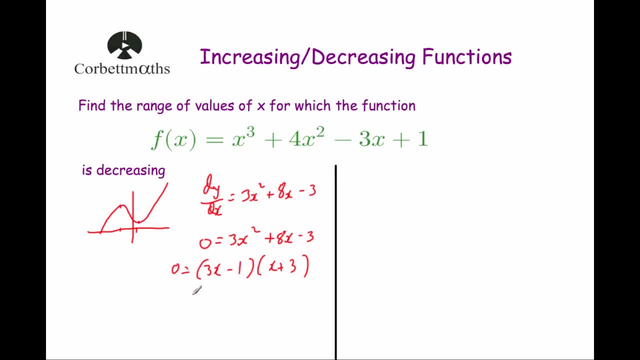 minus three, which is what we wanted. so let's find our values for x here. so x equals: here we are going to get one third, and here we're going to get x is equal to minus three. so that means that our, when we go back to our graph of our function, our first turning point will be at negative three. 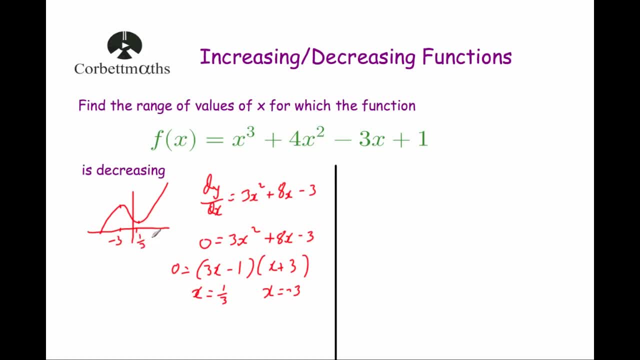 and our second turning point will be at one third. so we're trying to find when this function is decreasing. so it's for all the values of x in between minus three and one third. so let's write that down so that x is any value of x where that is bigger than negative three but less than one. 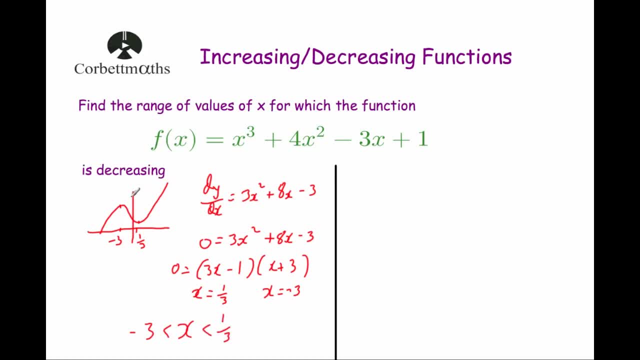 third will be a decreasing, or will give us a decreasing function. okay, so that's by considering those key points, those stationary points. the second approach is just by using the knowledge that if it's a decreasing function, that dy by dx is less than zero. so dy by dx. well, we've differentiated already, so dy by dx. 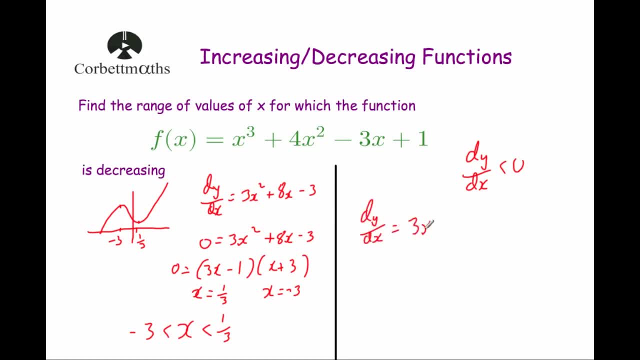 is equal to 3x squared plus 8x minus three, and we want to find when that is less than zero. so we're going to write that down: 3x squared plus 8x minus three is less than zero. now this is a quadratic inequality. to solve that, we're going to sketch the quadratic and our critical. 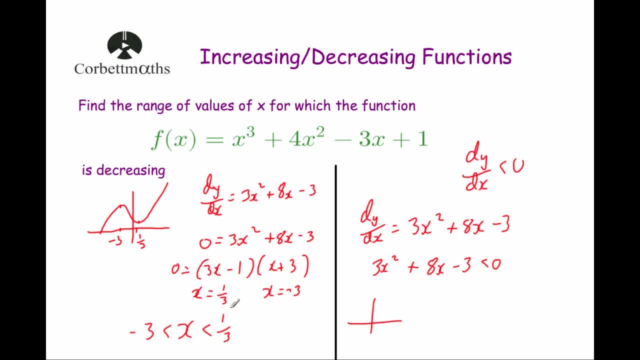 values. our points would be if we were to do this, we're going to do this, we're going to do this if we factorize this and solved it. well, we've already done that already. so we're factorizing it: 3x minus one and x plus three. so that would be here at negative three and here at one third. 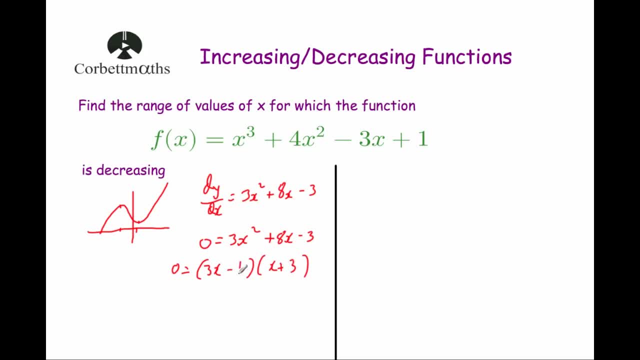 put a plus 3 over there, so that will give me 9x, and then a minus 1 here and let's just test that out. so we've got 3x times x is 3x squared. 3x times 3 is 9x minus 1 times x is minus x. that'll give me. 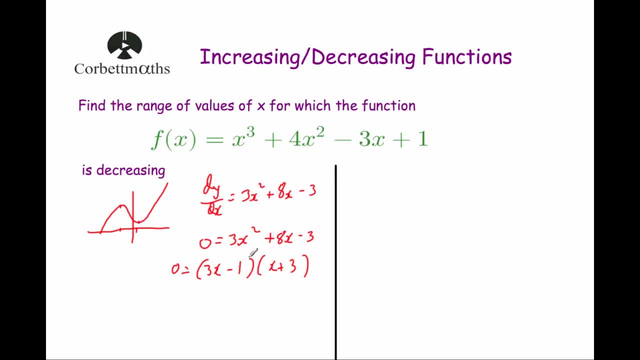 the 8x that we need, and minus 1 times 3 is our minus 3, which is what we wanted. so let's find our values for x here. so x equals: here we are going to get one third and here we're going to get x is. 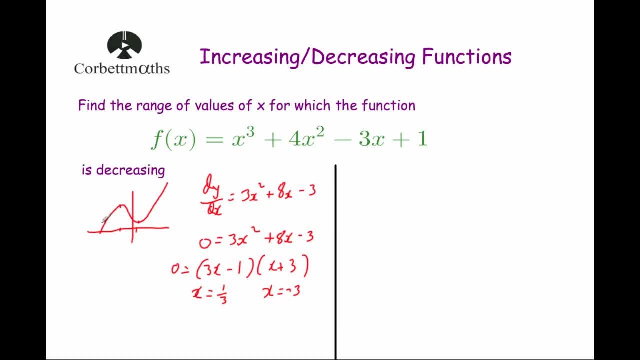 equal to minus 3.. so that means that our, when we go back to our graph of our function, our first turning point will be at negative three and our second turning point will be at- so we're trying to find when this function is decreasing. so it's for all the values of x in. 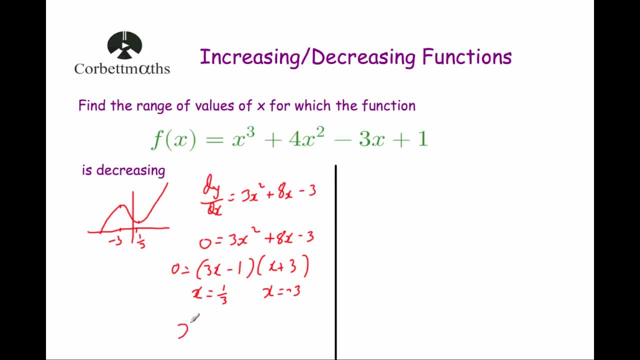 between minus three and one third. so let's write that down so that x is any value of x where that is bigger than negative three. but less than one third will be a decreasing or will give us a decreasing function. okay, so that's by considering those key points, those stationary points, the 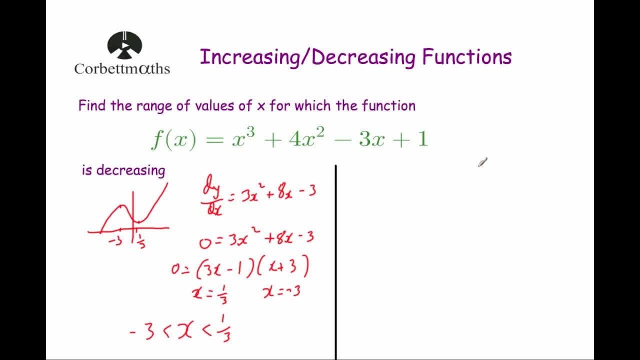 second approach is just by using knowledge that if it's a decreasing function, that dy by dx is less than one third. so dy by dx. well, we've differentiated already. so dy by dx is equal. so dy by dx is equal to 3x squared plus 8x minus 3, and we want to find when that is less than zero. 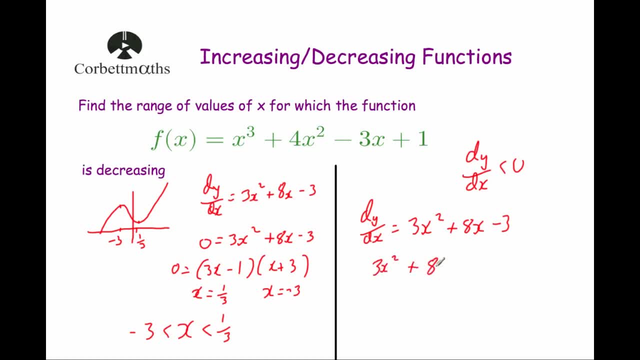 so we're going to write that down: 3x squared plus 8x minus 3 is less than 0.. now this is a quadratic inequality. to solve that, we're going to sketch the quadratic um our critical values. our points would be if we factorize this and solved it. well, we've already done. 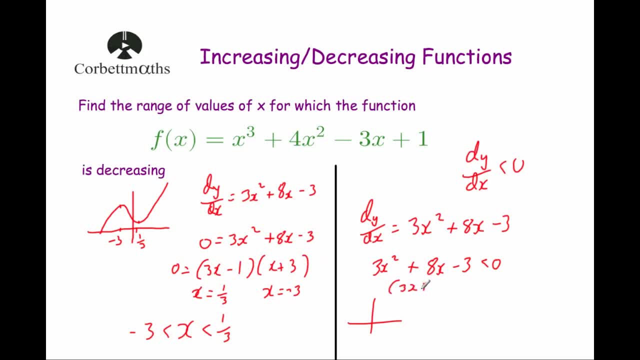 that already show you how best to solve that, but its just a bit out of the picture here, so ahead of time, i'll give you 10 as a non-modern uh des면 plotting. Rita already done that already. so factorizing it 3x minus 1 and x plus 3, so that would be here at. 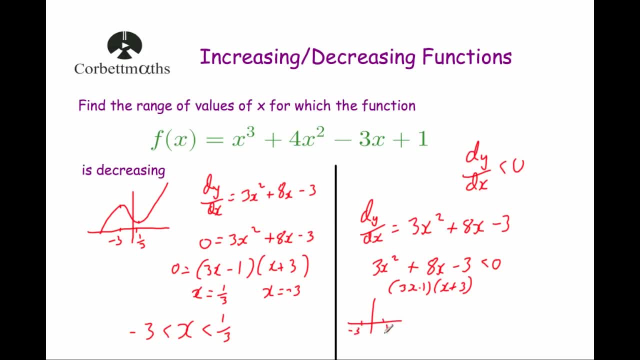 negative 3 and here at one third. and if we sketch that it would be, our quadratic would look something like that and we're trying to find when it's going to be less than zero. so that will be in between negative 3 and one third. so x will be less than one third but bigger than negative 3 and as you, 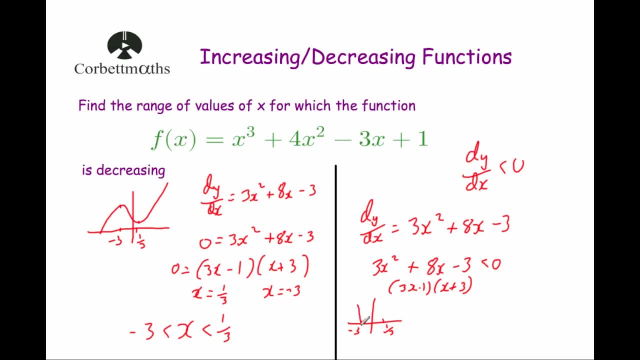 and if we sketch that it would be, our quadratic would look something like that and we're trying to find when it's going to be less than zero. so that will be in between negative three and one third. so x will be less than one third, but x will be bigger than negative three and, as you can see, both approaches give you the same answer. 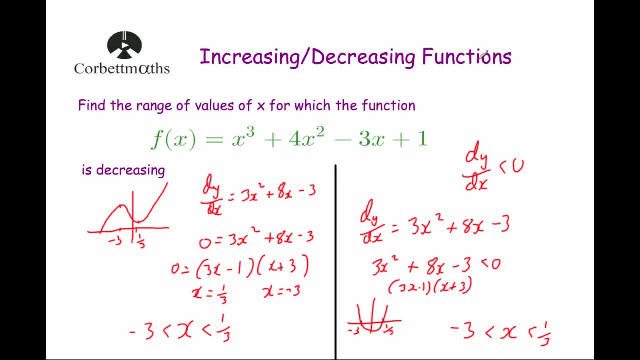 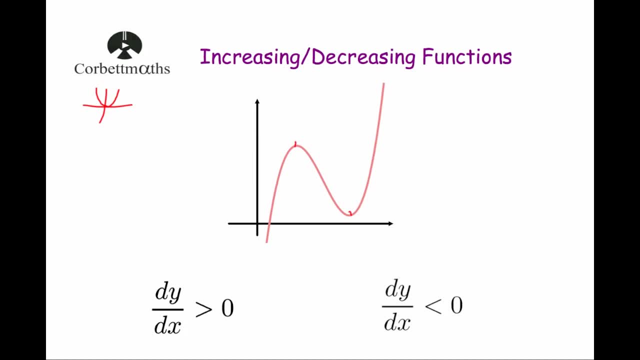 and that's it so for increasing and decreasing functions. obviously, if a function is increasing, dy by dx will be bigger than zero. if it's decreasing, dy by dx will be less than zero. some students prefer to solve this by considering what the graph or the function looks like, and 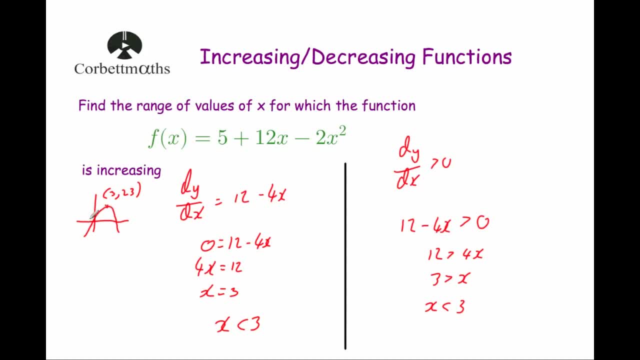 finding the stationary points and then using their common sense to work out when it's increasing or decreasing. and some students prefer to find the just if, get dy by dx and write down: it's bigger than zero, so that would be less than zero. so we're going to write that down and then we're going to. 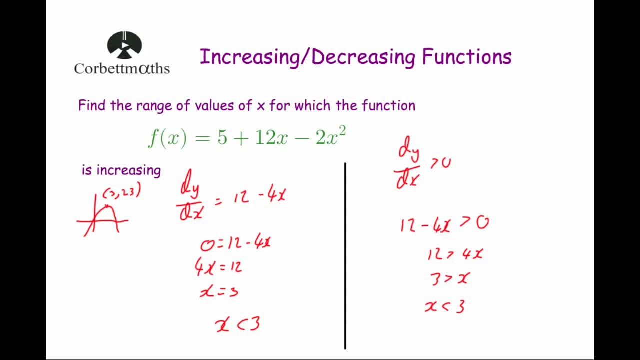 solve that inequality or less than zero, and solve that inequality, and that's it. and sometimes you'll get a quadratic and just remember how to solve quadratic inequalities, that's it. 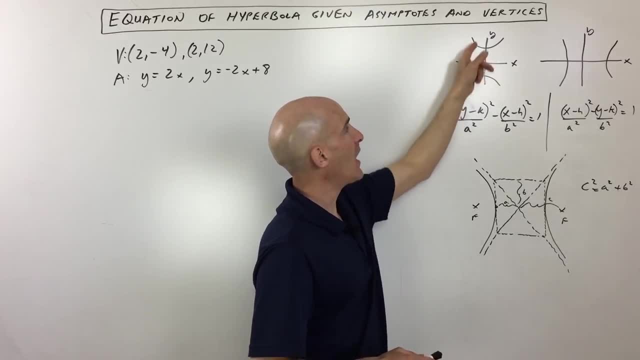 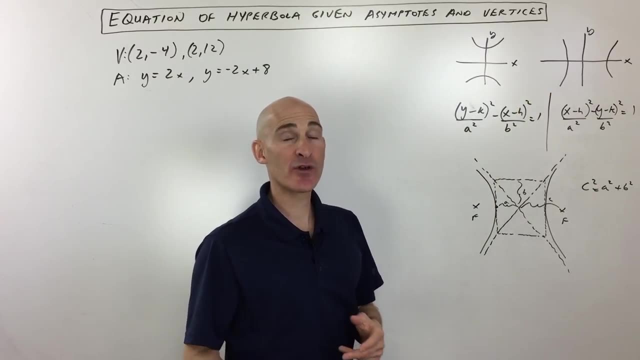 The main thing is with a hyperbola is that it's either going to be opening up and down, like in the y direction, or it's going to be opening left and right in the x direction. and if any of this seems confusing as I'm going through it, I'll have a link to another video I did talking about hyperbolas. 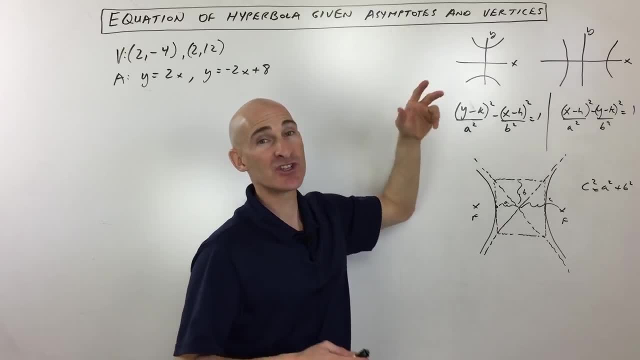 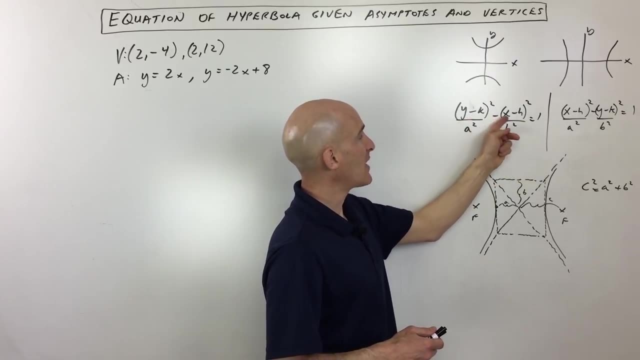 it goes into more depth. but this is a particularly challenging problem when they just give you the asymptotes and vertices. so I want to show you how to work with this one. but the basic equation you can see is: y minus k squared minus x minus h squared equals one and you've got your a squared. 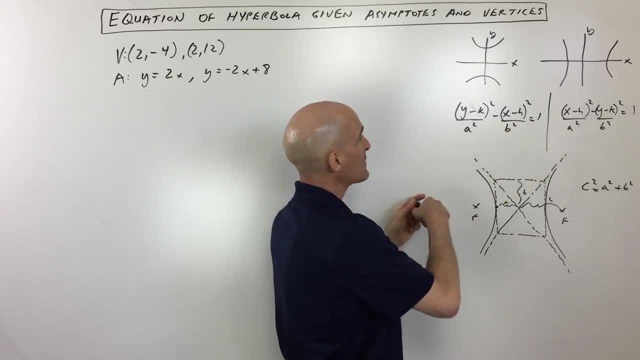 and your b squared. but the important differences here are that notice that here you've got the y squared as the positive term when the hyperbola is opening in the vertical direction, the y direction up and down, and here you've got the x squared as the positive term when it's opening in the 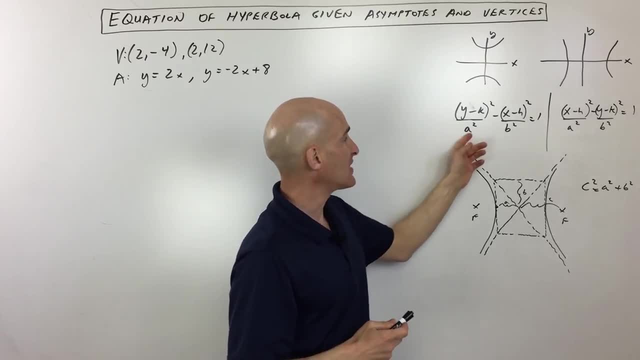 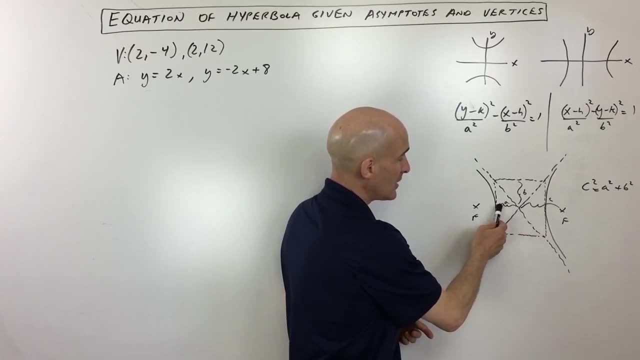 horizontal direction, in the x direction, left and right, and you notice that a squared is with that first term of that positive term. and then, just again, just to refresh, the distance from the center to the vertex, this point where the hyperbola bends or turns, that distance is a, the distance.